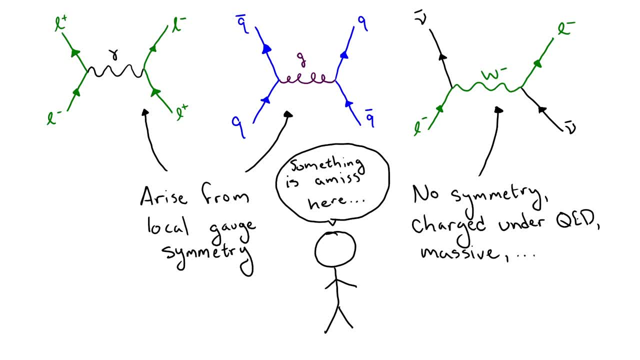 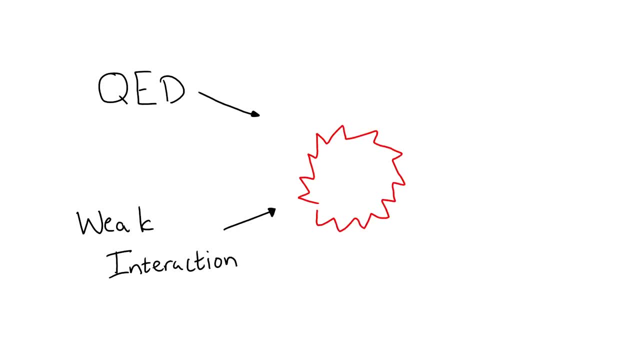 the gluons are only charged under their associated interaction of QCD. It turns out that this unpleasantness can be resolved in an interesting way: by unifying electromagnetism and the weak interaction into one combined force. This unification is known as electroweak theory, or sometimes the Weinberg-Solom model. 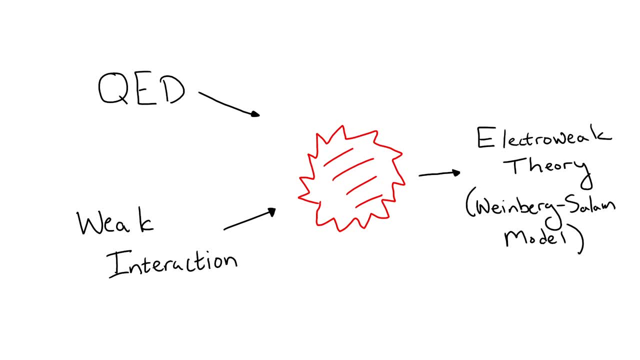 though the contribution of this unification can be found in the theory of the weak decays, In addition to the formulation of the theory from other physicists like Sheldon Glashow, Gerard et Hooft and John Ward, should not be understated. 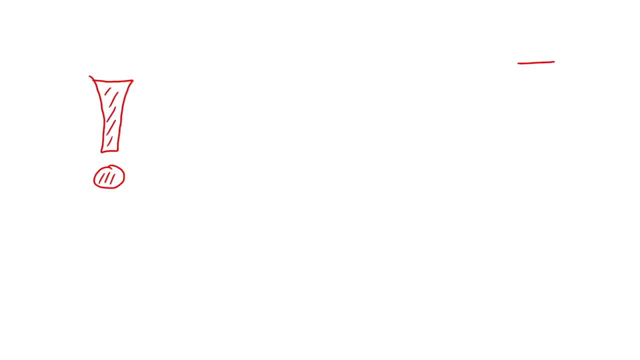 Now I do want to put a bit of a disclaimer on this video. Electroweak theory can be quite complex, even with some background in particle physics, so this video might get a little technical in places. I would highly recommend watching my other videos on the standard model. 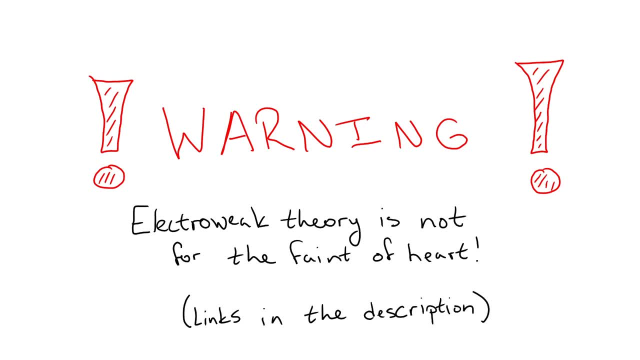 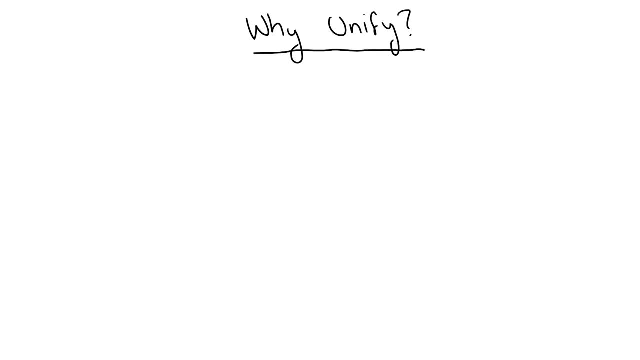 as well as spontaneous symmetry breaking first. if you haven't already, Okay, now it actually turns out that there are some good reasons to believe that the weak and the electromagnetic interactions should be unified. First and foremost, the W boson is massive. 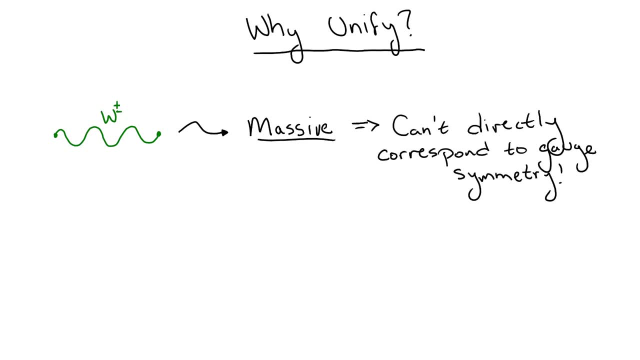 and so these particles cannot be directly tied to a conserved gauge symmetry, since a mass breaks such a symmetry. However, we also know that we can give gauge bosons mass by spontaneously breaking the associated local symmetry through the Higgs mechanism. So it's perfectly feasible that this massive W boson could arise from a spontaneously broken. 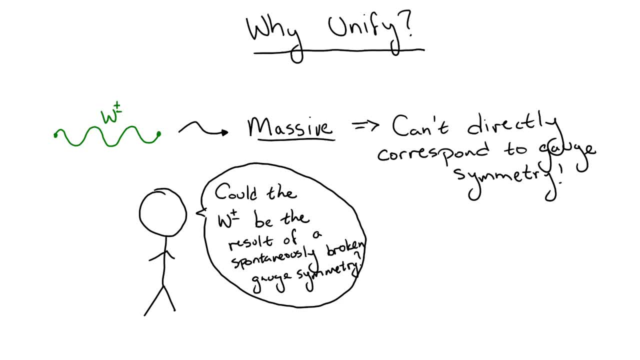 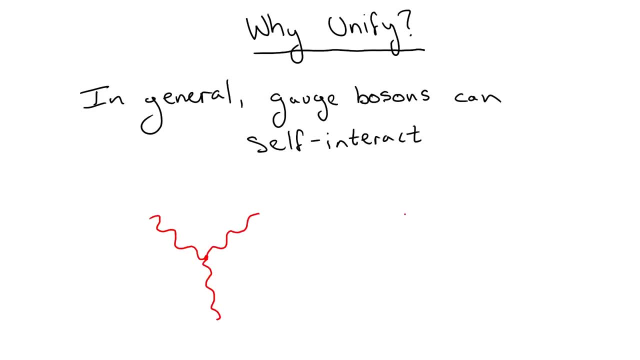 gauge symmetry. But how does this tie into electromagnetism? Well, to see this, we have to recall two things. First is that the gauge bosons corresponding to local symmetries can, in general, interact with themselves, In other words, they can be charged under their 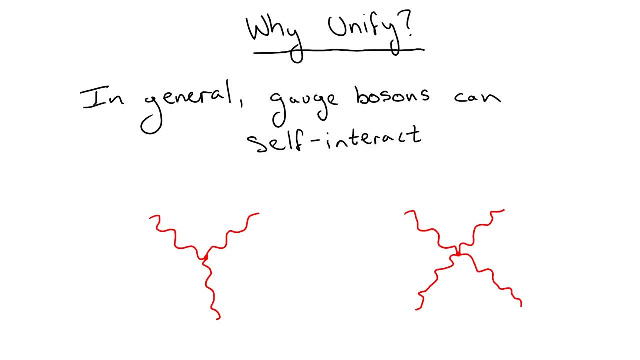 own interaction, just like we see in QCD. The other thing we need to remember is that when a symmetry is spontaneously broken, not all of the symmetries have to be broken. So after a gauge symmetry is spontaneously broken, some of the gauge bosons can remain massless. 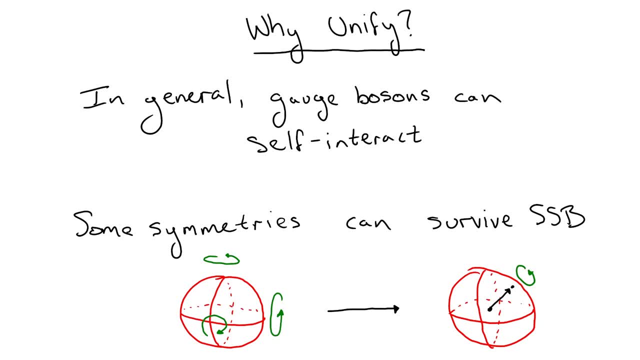 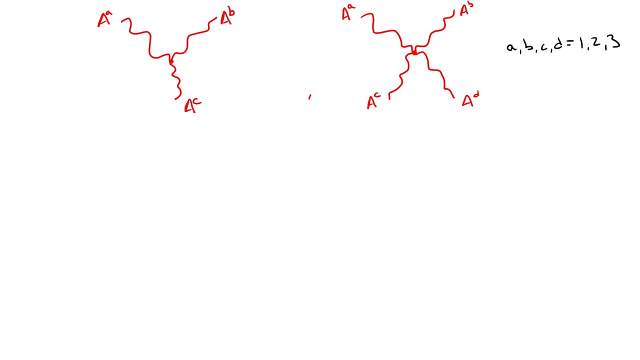 So let's combine these two ideas. Say that before spontaneous symmetry breaking our gauge bosons self-interact, But then we only partially break the symmetry so that some symmetries are preserved after the breaking. Then, due to the self-interactions, the 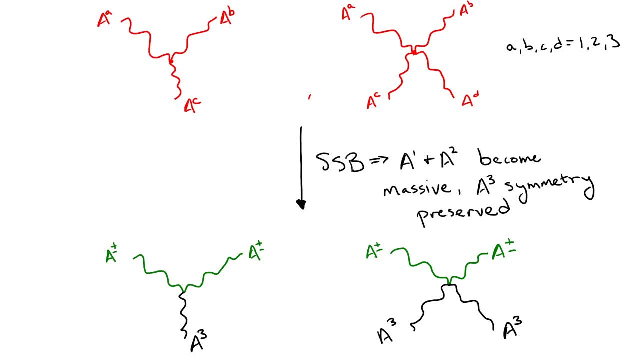 gauge bosons which obtain mass can interact with the massless gauge bosons of the preserved symmetry And therefore the massive bosons are charged under the preserved gauge symmetry, just the way the massive W boson is charged under QED. Clearly, by just considering the 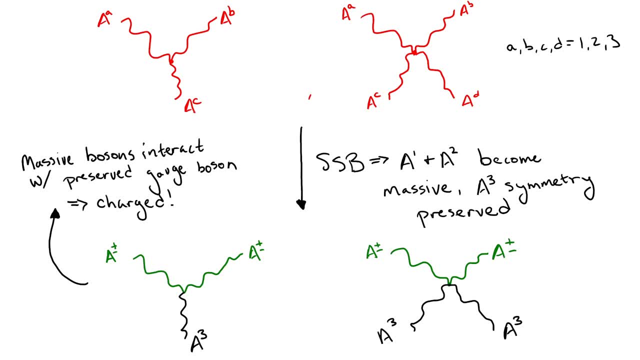 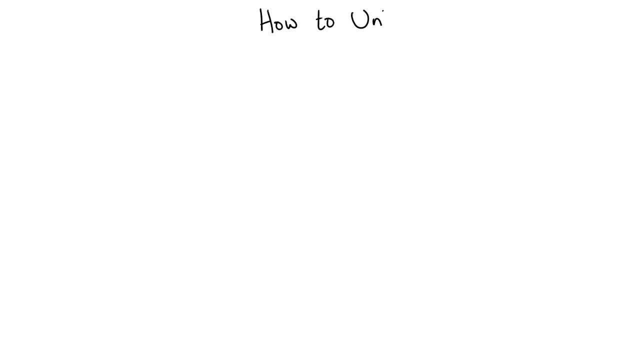 interactions of gauge bosons. it looks like we can unify the electromagnetic interaction and the weak interaction into some combined electroweak interaction. Now, how do we actually go about doing this? Based off of what we've already established, we can start building a checklist of the properties. 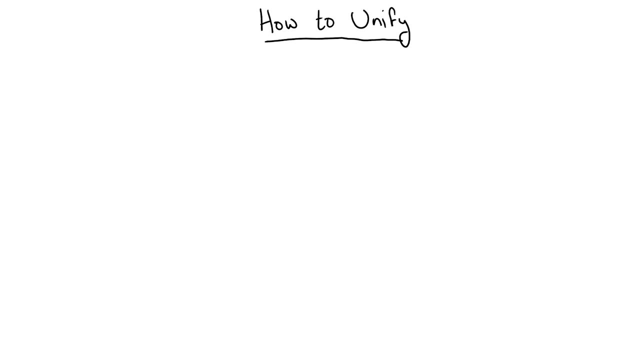 that we need this unified interaction to satisfy in order to be consistent with the physics that we observe. First, we need spontaneous symmetry breaking of a gauge interaction, which means that we not only need a gauge symmetry to break, but also a scalar particle that is charged under this. 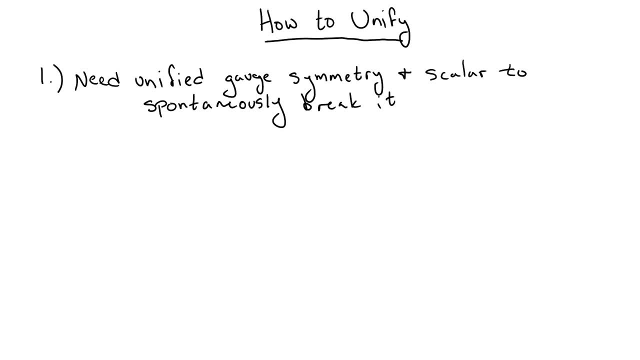 interaction which will induce the symmetry breaking. Second, once the symmetry is broken, we need a surviving symmetry. So we need a surviving symmetry to break the gauge symmetry which corresponds to QED and we need at least two massive gauge bosons. 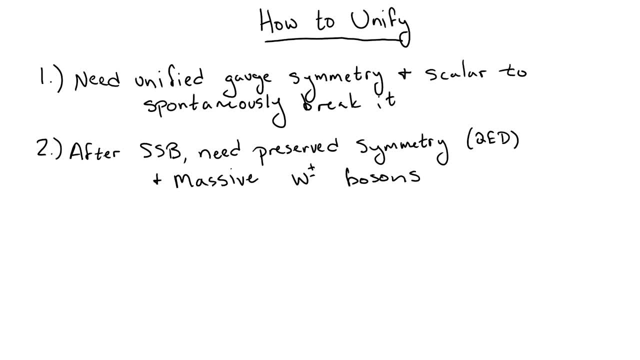 which correspond to the W plus and W minus. Third, the gauge symmetry needs to feature self-interactions between gauge bosons in order to produce a charged W boson after symmetry breaking. Now, this checklist isn't done yet. We still need to consider what is happening with the 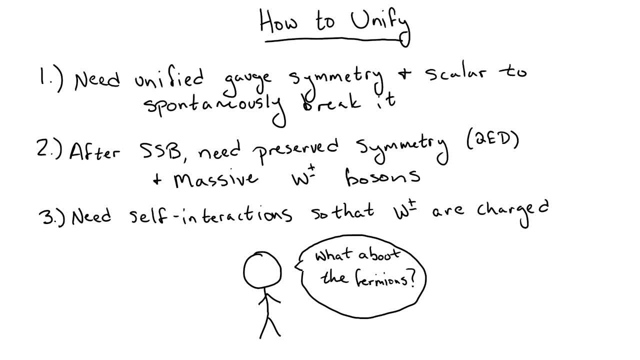 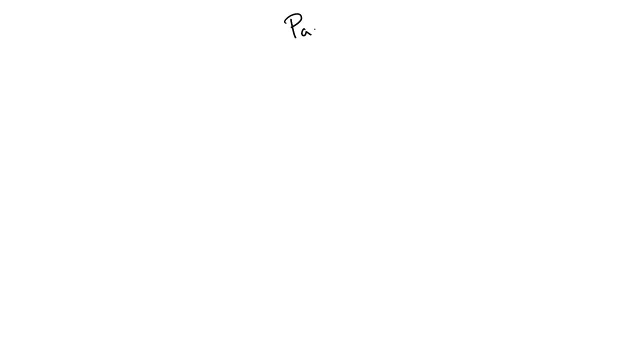 fermions in the theory and, as it turns out, the weak interaction actually has quite an interesting relationship with these fermions. To understand this, we have to revisit the concept of parity. Recall that parity is defined as the transformation which flips all spatial axes. 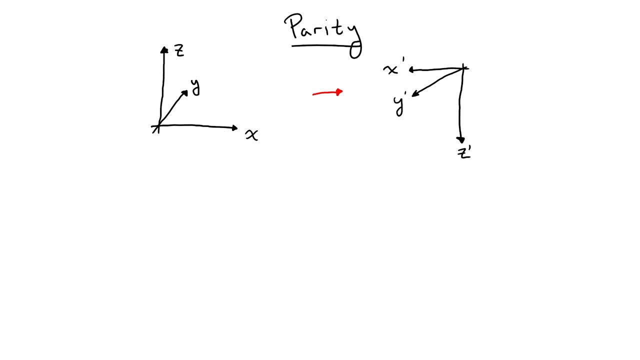 and importantly, different mathematical objects change in different ways under such a transformation. In this case, the fermions that we've been talking about are described by mathematical objects known as spinners. Interestingly, there's not just one type of spinner. In fact, up to this point in the series, we've secretly been restricting our 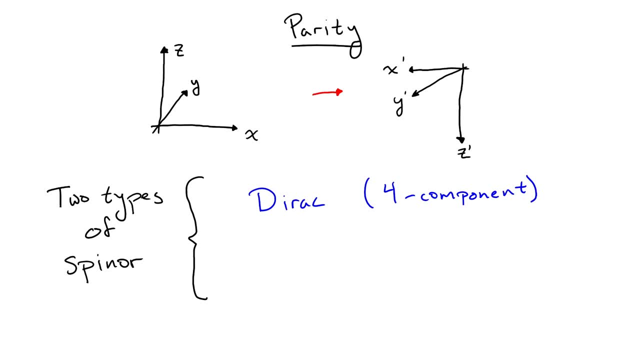 discussion to so-called Dirac or four-component spinners. These are convenient when we use parity symmetric theories such as QED and QCD. but there's another type of spinner, known as a Vial spinner or two-component spinner, which becomes necessary to talk about when working. 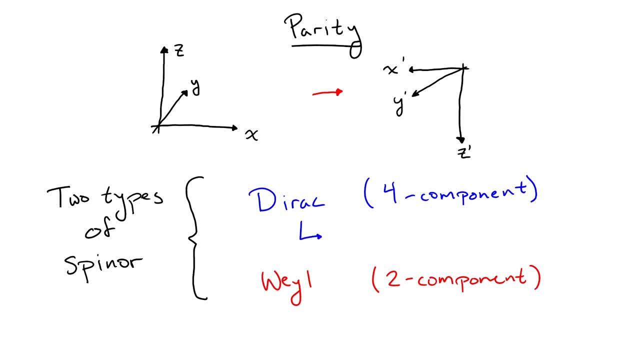 with the weak interaction. In fact, Dirac fermions can really be thought of being made up of two vial fermions, typically given the names of left- and right-handed components. These components actually transform differently under Lorentz transformations as well as under parity. 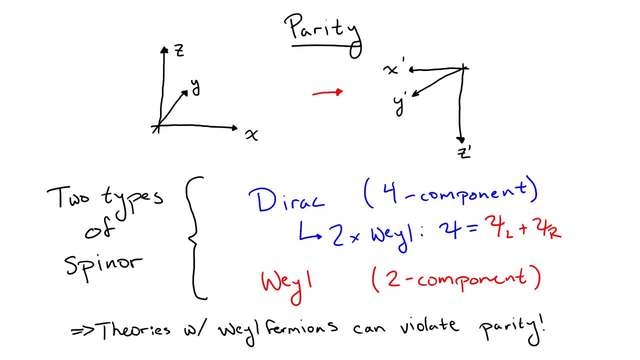 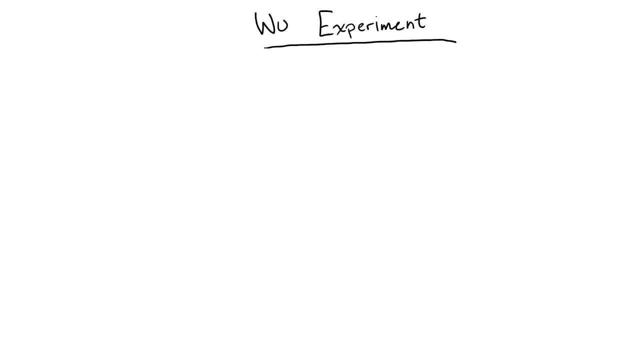 meaning that we can feasibly build parity-violating theories using these vial spinners. So why does this matter? Well, as it turns out, an experiment conducted in 1956 by Xianxiong Wu proved that weak decays do not conserve parity. 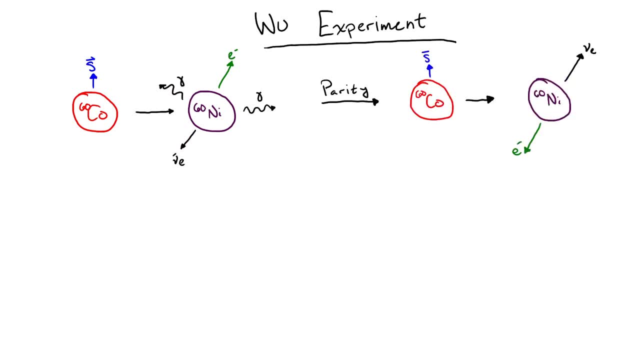 Famously, Wu did not win a Nobel Prize for this groundbreaking discovery, but her collaborators TD Li and CN Yang did. This fact tells us that the weak interaction does not equally talk to the right- and left-handed components of the fermions in the standard model. 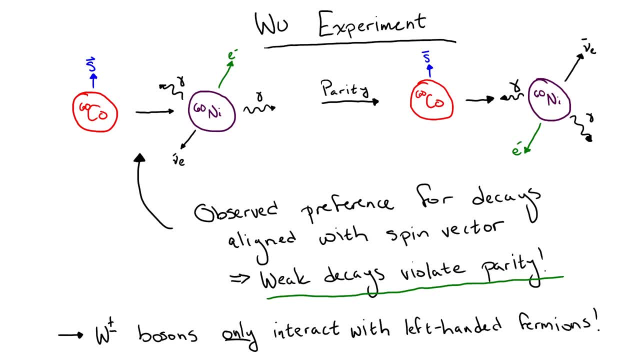 In fact, the W boson only interacts with the left-handed pieces. This means that if we want to unify electromagnetism and the weak interaction into a unified game, then we have to use the weak interaction to unify electromagnetism and the weak interaction into a unified game. 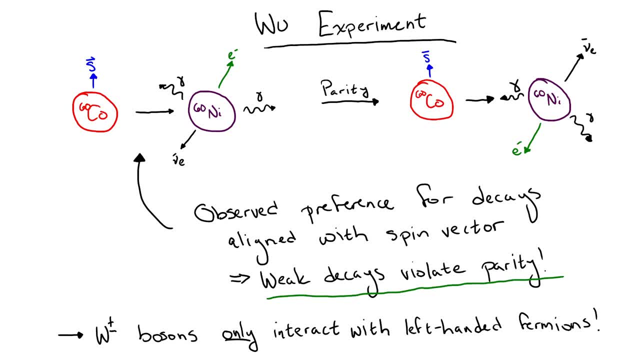 For example, if we want to unify electromagnetism and the weak interaction into a unified game, then we have to use the weak interaction to unify electromagnetism and the weak interaction into a unified game. This interaction should treat left- and right-handed components of fermions differently. 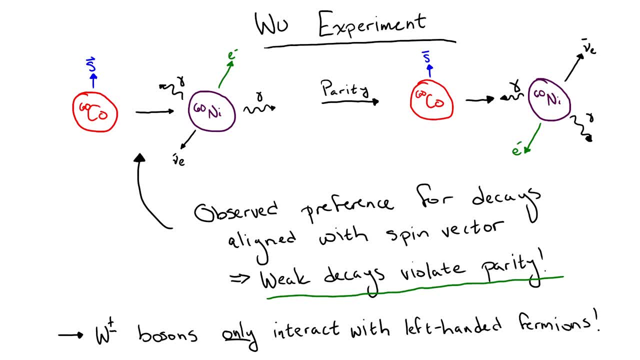 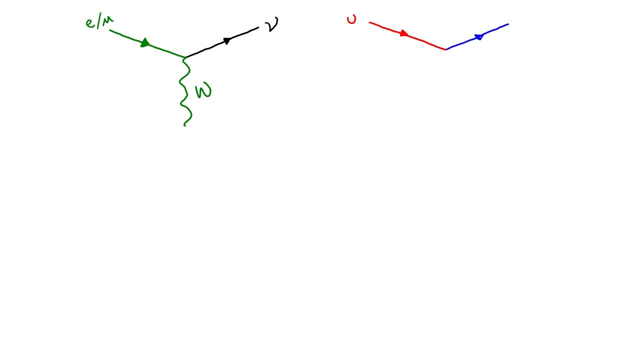 What we do know is that we can achieve the same result by using the weak interactions of the fermions. Such a theory is typically known as the chiral gauge theory, But this still isn't the end of the story. We also know that fermions are, quote unquote, paired up according to their weak interactions. 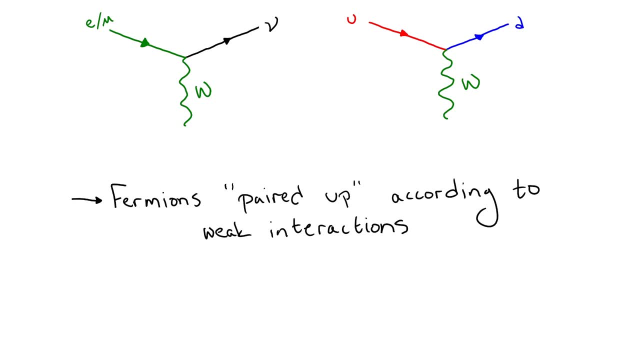 In particular, we saw that the up quarks are paired with the down quarks and the charged leptons are paired with neutrinos. So are you sure that you can solve the problem if you are not a quark? If you are, then you are right. 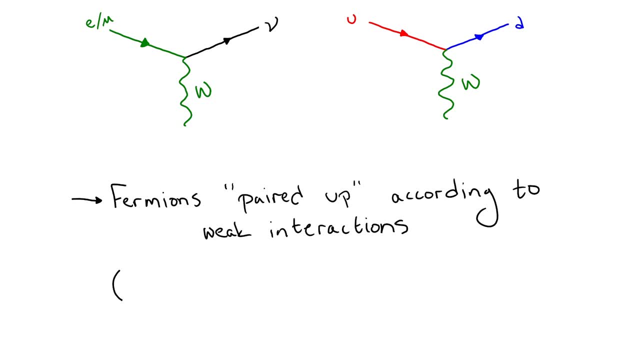 If you are, then you are right. So our unified interaction should reflect this feature and shouldn't introduce any new pairings between, for example, up quarks and charged leptons. Finally, since most of the fermions that we have discussed are massive in the standard model, 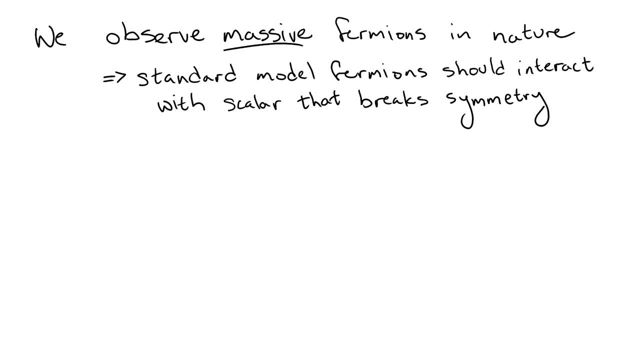 we need a way to generate couplings between these fermions and the scalar, which spontaneously breaks the symmetry. As it turns out, this introduces an added complication. Two-component spinners which are charged under a gauge symmetry cannot be massive by themselves. Such a mass term would explicitly break the gauge symmetry. 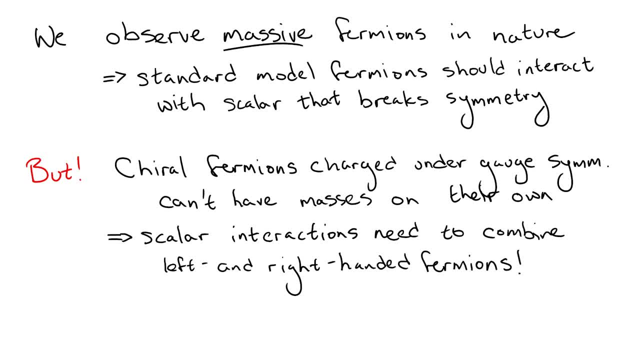 However, left- and right-handed components can be paired together to form so-called Dirac masses. So we know that the interactions with the scalar field, before symmetry breaking, must pair together left- and right-handed fermions in order to generate Dirac masses. 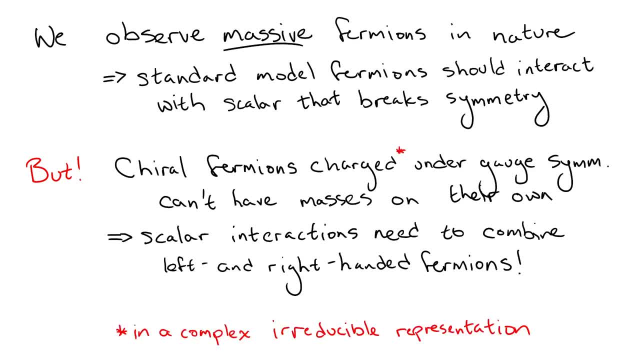 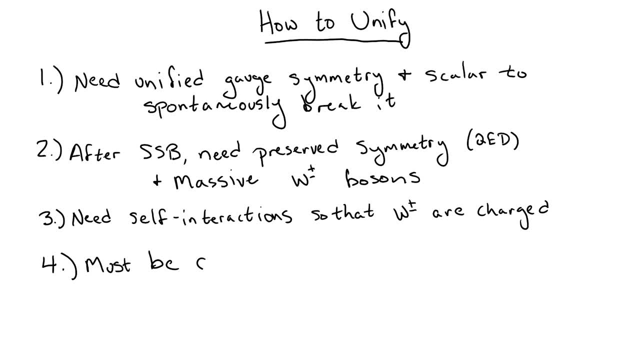 after the symmetry breaking. So we need to add the following items to our checklist in order to build the theory of electroweak interactions. This theory needs to be chiral and treat the left- and right-handed fermions differently. We need a way to combine pairs of fermions which participate together in weak decays. 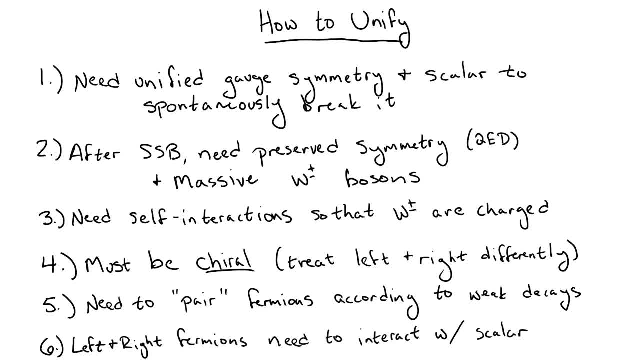 And the fermions must interact with the scalar. that breaks the symmetry in a way which produces Dirac masses after symmetry breaking. Alright, with this checklist, let's get to it: building our theory. Perhaps the easiest place to start is to guess at what gauge interaction 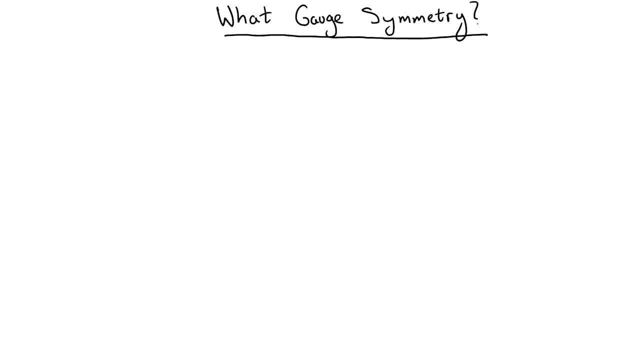 we actually need. Since we know that we need self-interactions of gauge bosons, we may suspect that we should have a theory similar to QCD, where the interacting particles have several charges under the gauge symmetry instead of just one, like we see in QED. 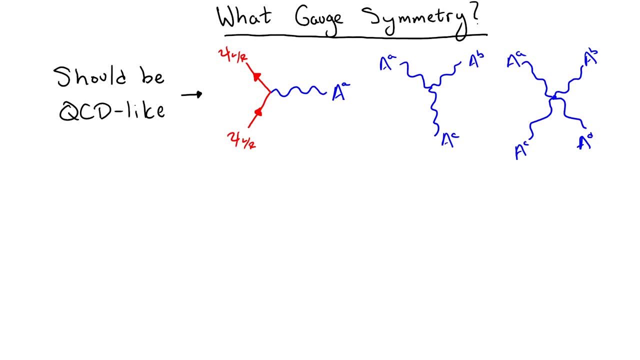 Now, as we saw in my spontaneous symmetry breaking video, when a gauge symmetry is broken, we don't lose or gain any gauge bosons, just some of them obtain a mass. This means we need at least three gauge bosons in our unified theory in order to form the two charged states of the W. 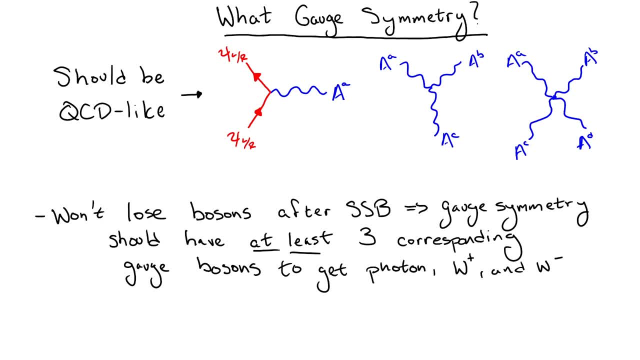 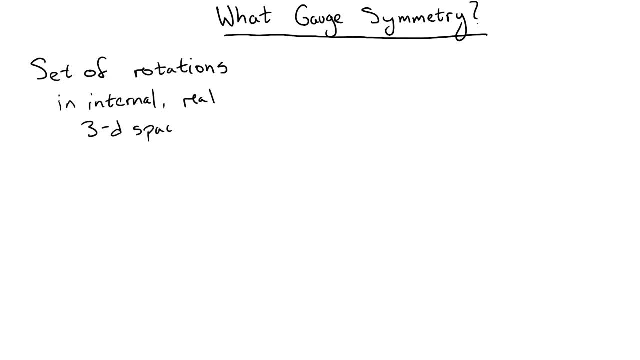 as well as the photon Recalling, that we get one gauge boson for each unique symmetry transformation. let's start off simple by considering symmetries which only have three unique transformations. One possibility is the set of rotations in rotation. If we have a set of rotations in rotation, we have a set of rotations in rotation. 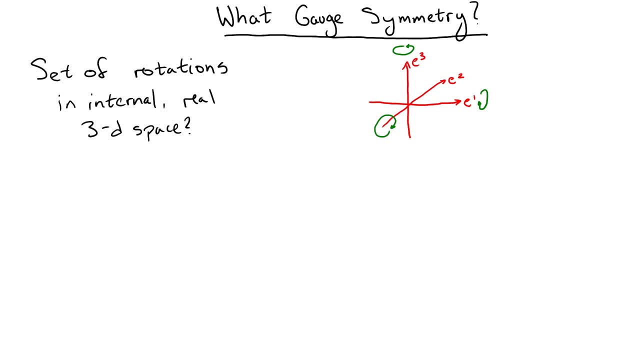 If we have a set of rotations in rotation. we have a set of rotations in rotation If we have real three-dimensional space which gives us one transformation in each of the three unique planes. As a note, remember that these are not physical spacetime rotations. 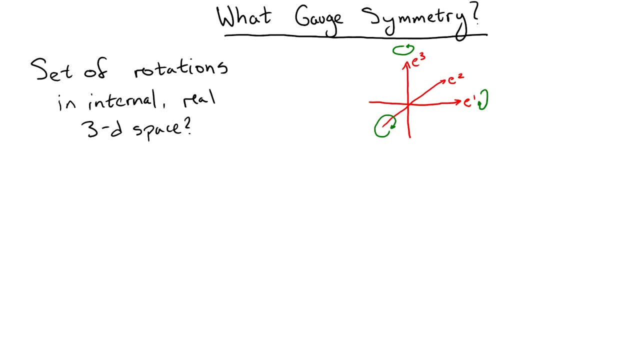 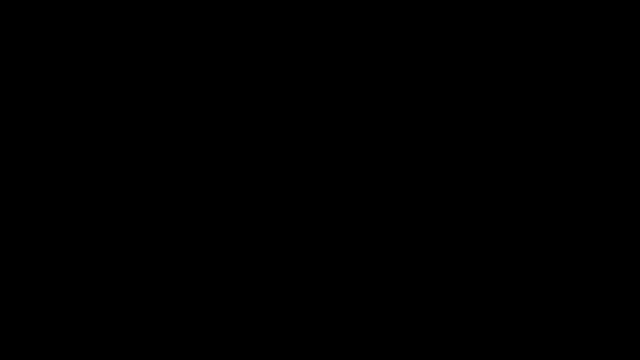 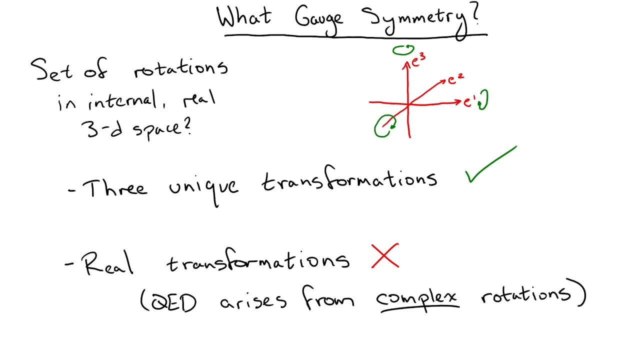 they are rotations on a real internal space which corresponds to the given gauge symmetry. Now, while this is a good first guess, it doesn't work due to the fact that we know that QED arises from complex internal rotations which we can't get from a set of real rotations. However, we aren't out of luck. 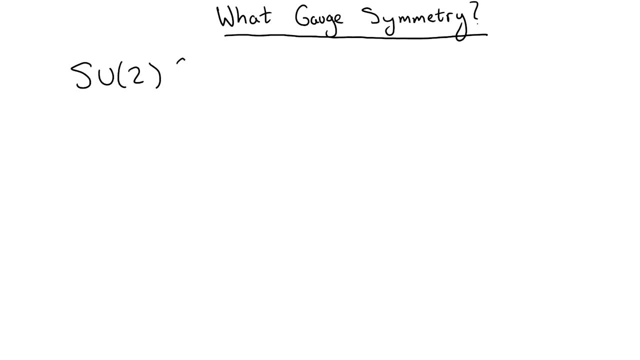 There is another group of transformations known as SU that has three unique elements which are complex. Here the SU stands for special unitary and just tells us that the transformations have to satisfy certain properties to fit in the group. The 2 tells us that the fundamental objects that 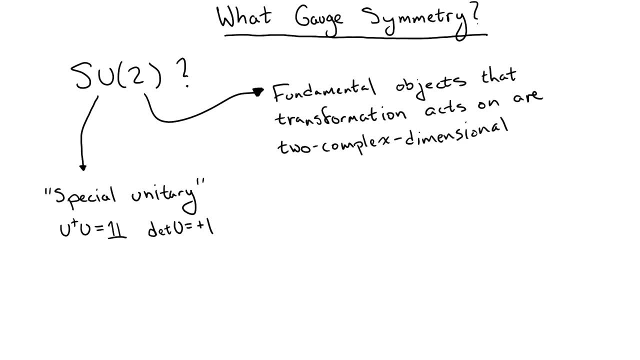 these transformations can act on are too complex-dimensional. So let's look at some of these transformations and see if we can find a way to solve them. This is actually quite nice. Recall that we need to pair up the fermions according to their weak. 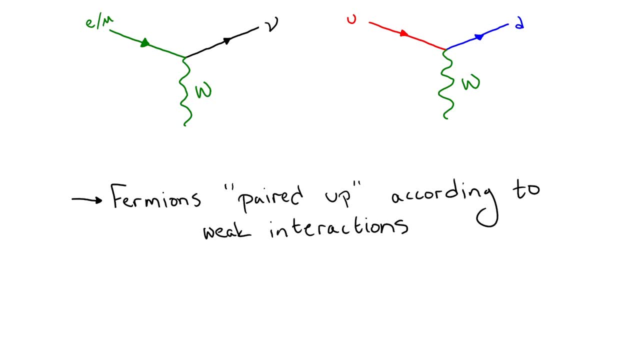 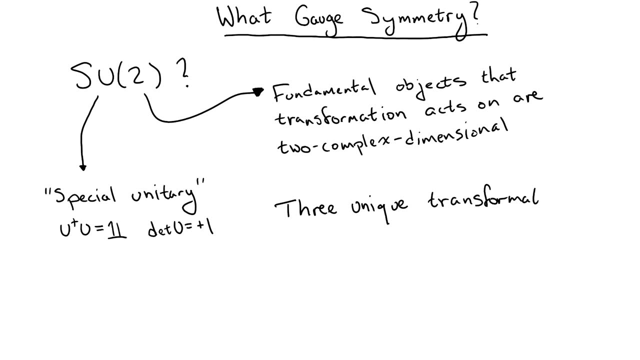 interactions. If the fundamental objects that these local SU transformations act on have two components, then we can simply place the fermion pairs into so-called doublets, which transform under this new gauge interaction. These two elements of the doublets are analogous to the three color charges of the quarks. 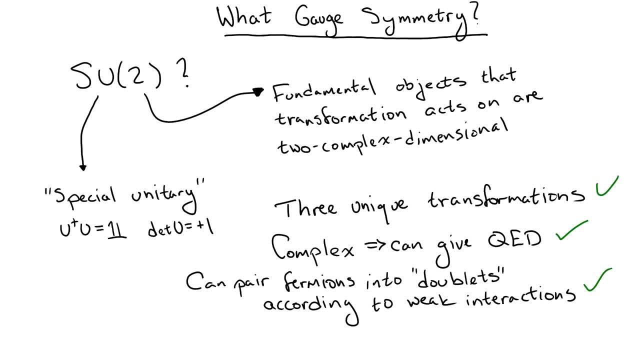 under this new gauge interaction. These two elements of the doublets are analogous to the three color charges of the quarks under the new gauge interaction. The second and final parameter is a new gauge interaction, and this new gauge interaction is called the qcd-sq2-sq2-sq2-sq3-qcd-qcd-qcd-qcd-qcd-qcd-qcd-qcd-qcd-qcd-qcd-qcd-qcd-qcd-sq3-qcd-qcd-qcd-qcd-qcd-qcd-qcd-qcd interaction. 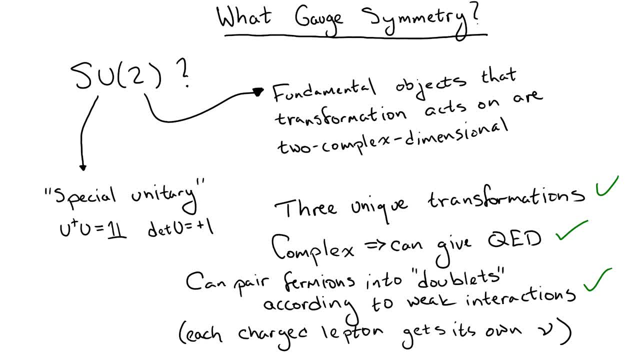 This means that we need to have one separate neutrino to pair with each charged lepton In this series. so far we've only talked about the electron and the muon, so we will include two neutrinos, known as the electron neutrino and the muon neutrino. So this SU gauge interaction seems to. 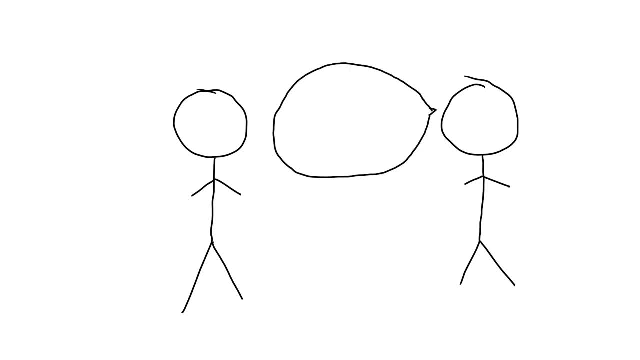 the unified electroweak theory, but we still haven't addressed all of the elements on our checklist, Namely, we haven't turned this into a chiral theory and we haven't found a way to give the fermions masses through scalar interactions. It turns out that we run into some problems here. 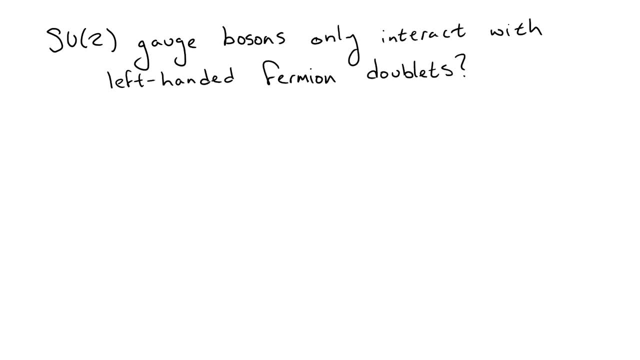 Since we know that the W boson will only talk to left-handed fermions after spontaneous symmetry breaking, we might be tempted to say that the SU2 interaction needs to only interact with left-handed fermions. But we have to keep in mind that on top of weak decays, we also have to reproduce QED, which is a parity symmetric theory, and we can't get this from just left-handed interactions. On top of that, if we want a scalar that will spontaneously break only SU2 to the one complex dimensional rotations of QED, we have to keep in mind that we also have to reproduce QED. 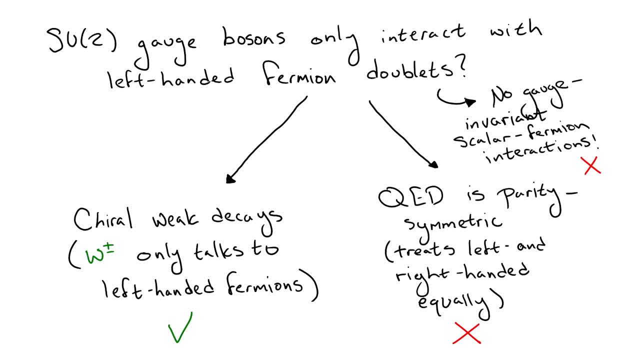 on top of weak decays, which is a parity symmetric theory, and we can't get this from just left-handed QED. It turns out that there's no way to write down interactions with the fermions and the scalar which will generate a mass term, at least at the renormalizable level, So it seems that we are part. 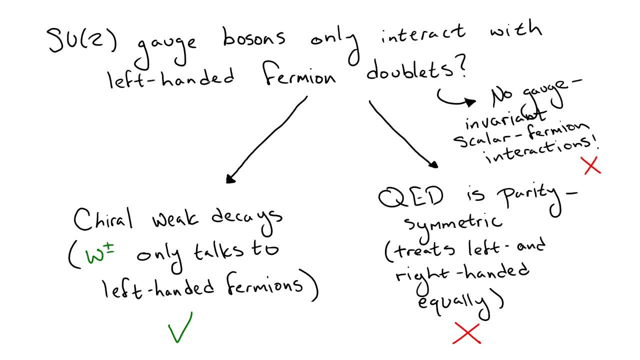 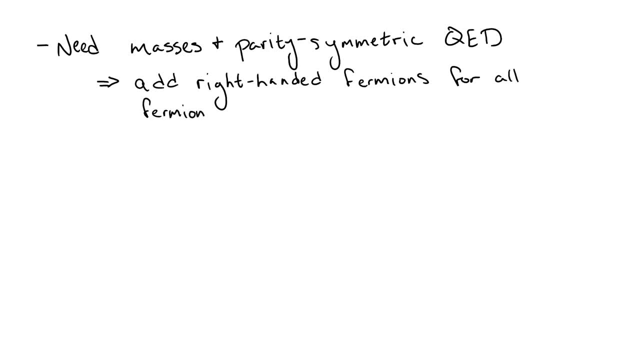 of the way there, but we still need to add something else to make everything work out. We still need to include right-handed fermions in order to generate both parity symmetric QED interactions as well as Dirac masses. So we will add one right-handed. 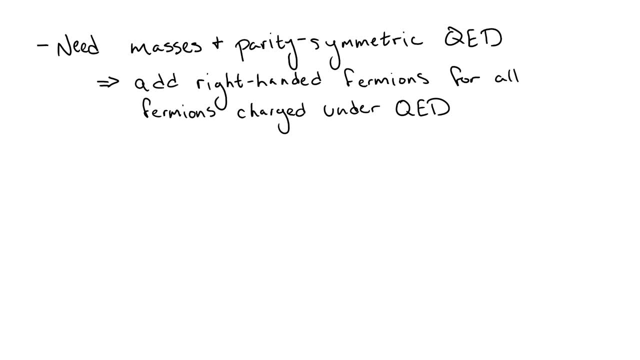 fermion, for each fermion, we know, is charged under QED after spontaneous symmetry breaking. Notice that this means that we do not add any right-handed neutrinos. They're not necessary for considering QCD since they're electrically neutral and since they only interact via the 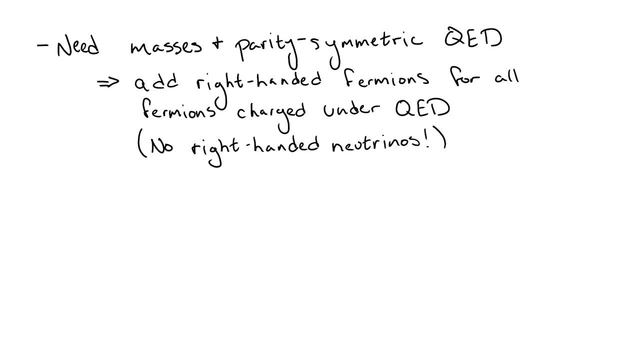 weak interaction. only left-handed neutrinos have been experimentally observed. The consequence of this is that we can't add a Dirac mass for the neutrinos and therefore they are massless in the standard model. Now we will maintain the SU2 interaction. 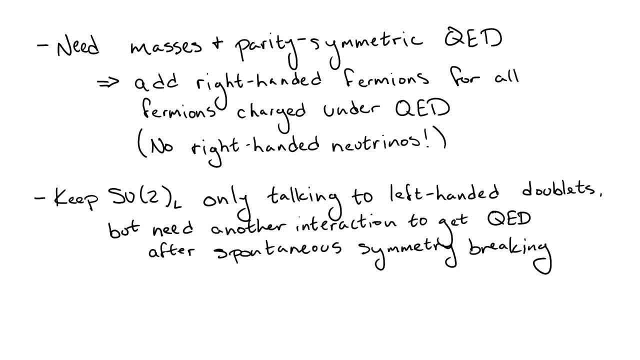 so that it only interacts with the left-handed fermions in order to keep the parity violation of weak decays, But we need to introduce an additional interaction that talks to the right-handed fermions as well as the left-handed ones, in order to reproduce QED In the interest 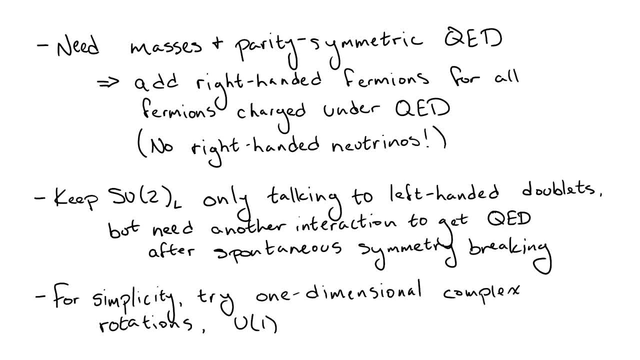 of keeping things minimal, we will simply include a gauge symmetry corresponding to one complex dimension. The name of the group of these rotations is U1, where again the U stands for unitary and the 1 tells us that the rotations act on one complex dimensional object. 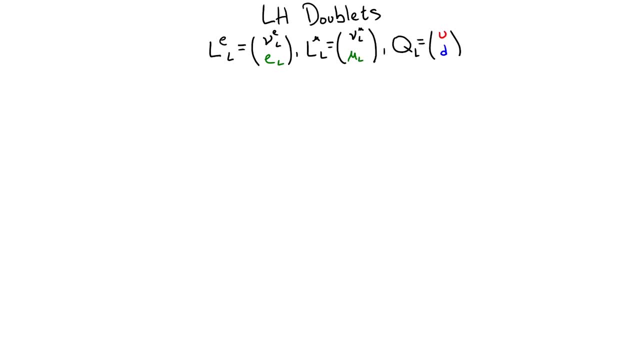 So we have an SU2 gauge interaction, which acts on the left-handed fermions only, with associated gauge bosons called the W1, W2, and W3, as well as a U1 gauge interaction with only a single gauge boson called the B, which interacts with both the 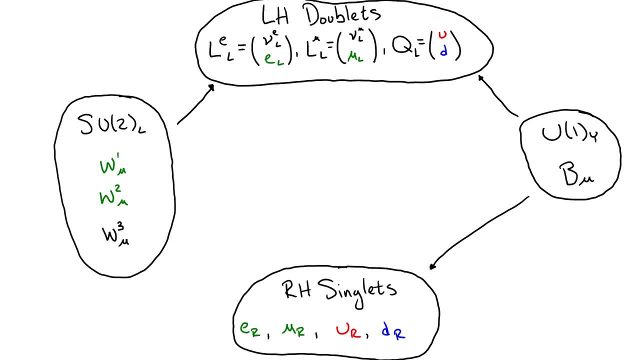 left-handed doublets as well as the right-handed singlets. The charge of a field under the SU2 is typically known as weak isospin not to be confused with the isospin symmetry of the strong interaction, and is denoted as τ3.. 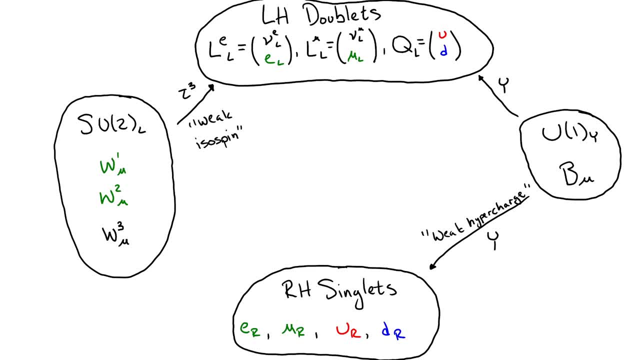 And charge under the U1 is known asulk hypercharge and is denoted with a integration y. After working through all of the math, it turns out that this combined gauge symmetry can be spontaneously broken by a scalar field which transforms as a doublet under SU2 and has 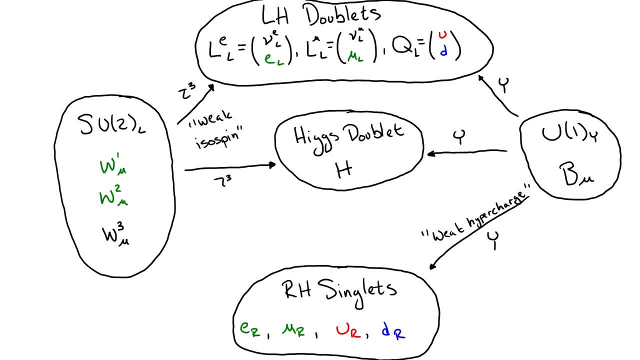 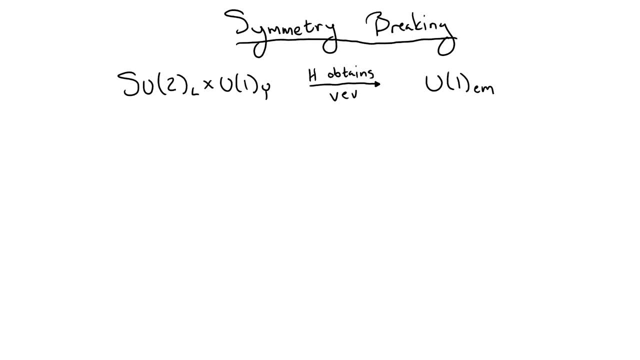 non-zero hypercharge called the Higgs doublet. Once this symmetry is broken by such a Higgs doublet, there's a leftover parity symmetric U1 gauge symmetry, which we can identify with quantum electrodynamics just as we wanted. A couple of interesting things happen when this 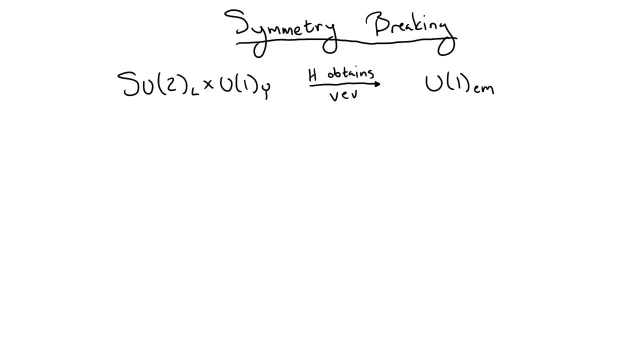 symmetry is spontaneously broken While some of the gauge bosons become massive. they're also mixed together into linear combinations. The W1 and W2 mix in two different ways to form the two charge states of the massive W boson, and the W3 and B bosons mix together to form the massless. 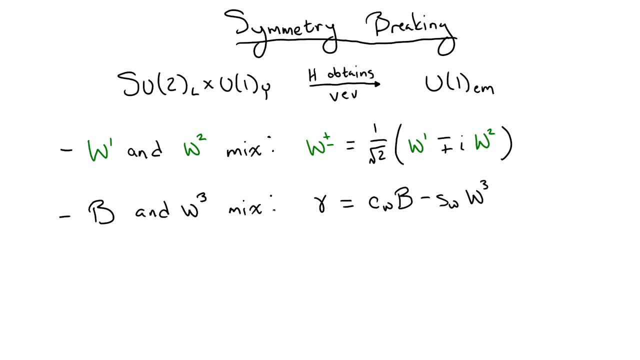 photon corresponding to the remaining gauge. This mixing also has the consequence of combining the weak isospins and hypercharge of the other particles in the theory to form their electric charge. Amazingly, the particle content that we've included so far allows us to combine the Higgs doublet as well as left-handed doublets. 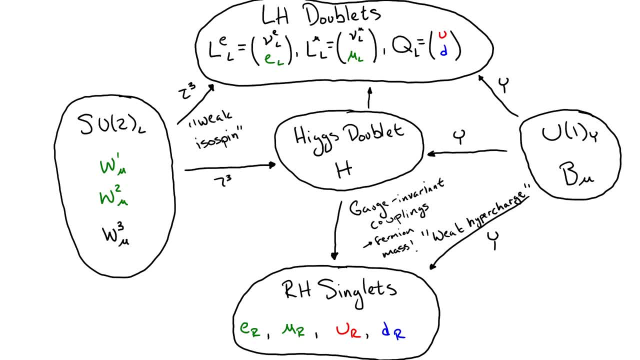 and right-handed singlet fermions and to gauge invariant interactions which produce fermion masses after symmetry breaking. Let this sink in for a second. The hypercharges and weak isospins of all of these particles are fixed by both group theory and the requirement that they combine to produce the correct electric. 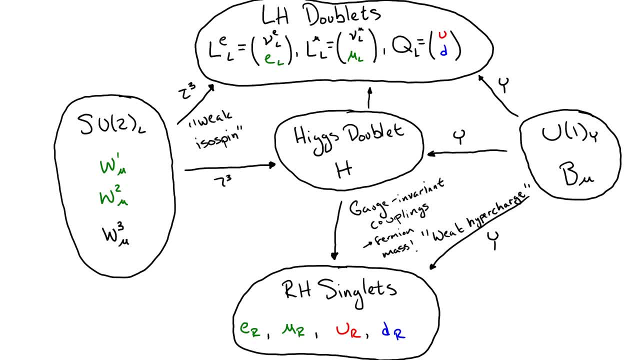 charge of the particles after symmetry breaking. It just so happens that these quantum numbers perfectly work out when combined to form such mass terms which preserve electroweak gauge symmetry. This is just one example of how perfectly the electroweak theory fits with the reality. we 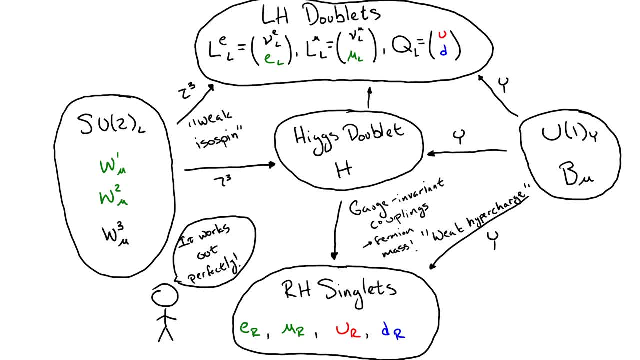 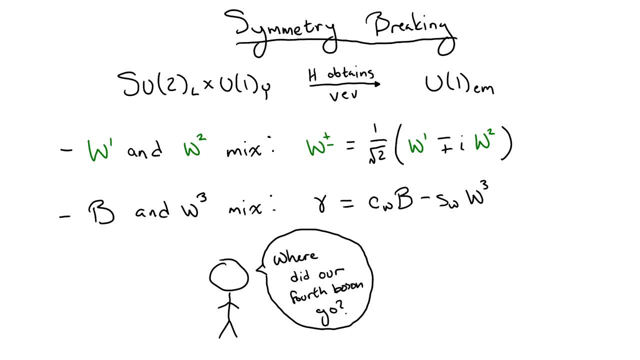 observe, But we still aren't done. Remember that we don't lose any gauge bosons from spontaneously breaking a symmetry. But before symmetry breaking we had four gauge bosons: the three w's and the one b, But after symmetry breaking we only have three: the w plus and minus, and 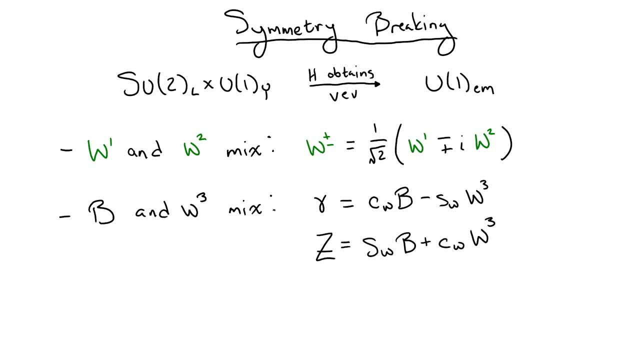 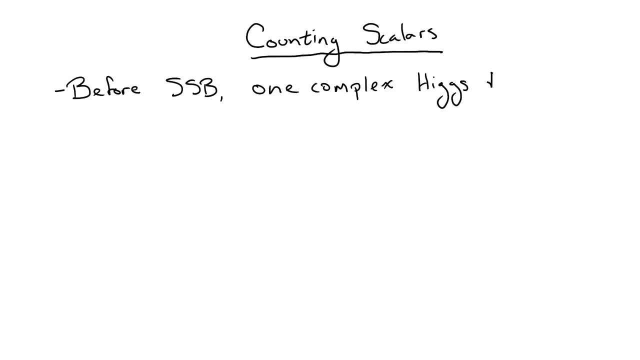 the photon. There is, in fact, an additional way of mixing the w3 and b gauge bosons other than the photon, and this leads to an electrically new theory. Before symmetry breaking, we have a single Higgs doublet which has two complex elements. 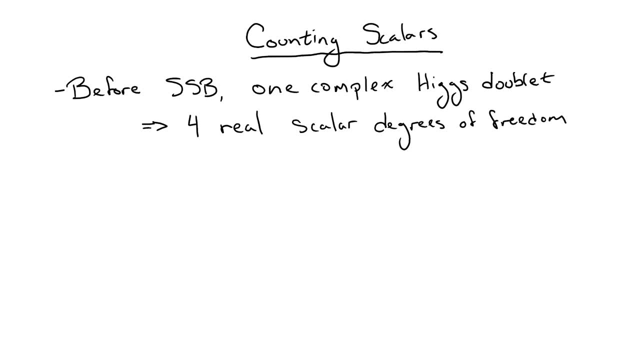 or four real elements, As explained in my video on spontaneous symmetry breaking. whenever a symmetry is spontaneously broken, we get one goldstone boson, four real elements. In this case, we have four unique symmetry transformations before breaking and only one after. 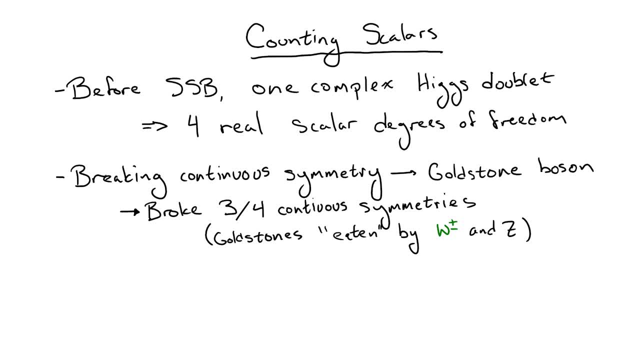 So we need three goldstone bosons. These goldstone bosons are eaten by the w plus and minus and z gauge bosons in order for them to obtain a third transverse polarization once they become massive. So we should have one left-over real scalar degree of freedom which is massive and neutral. 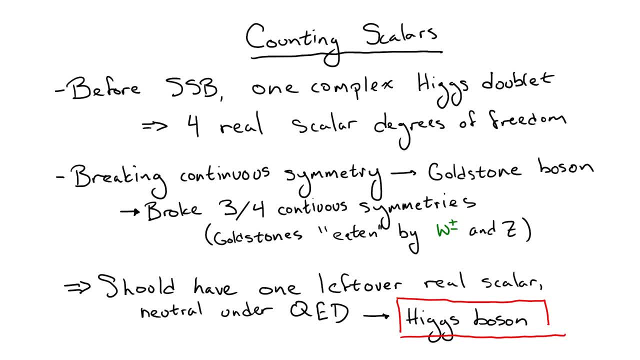 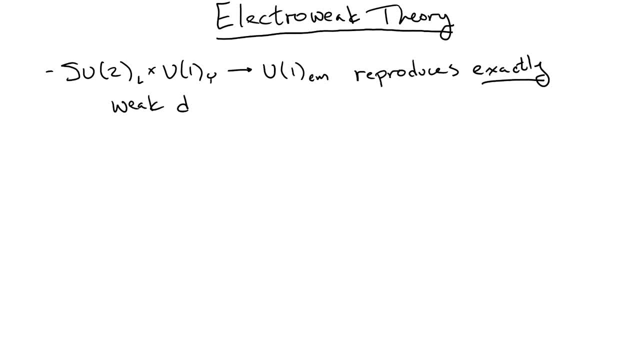 So we have one left-over real scalar degree of freedom which is massive and neutral under electromagnetism. This particle is known as the Higgs boson. Notice that not only is this theory reproducing exactly what we see physically in terms of 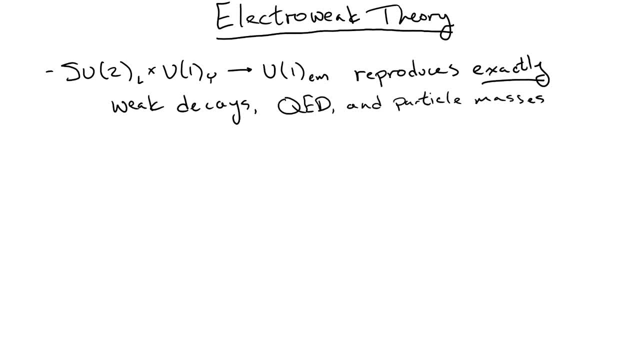 QED and weak decays, as well as generating masses for the gauge bosons and fermions. it's also predicting the existence of two particles which are absolutely necessary for the theory to be valid, namely the z and the Higgs bosons. 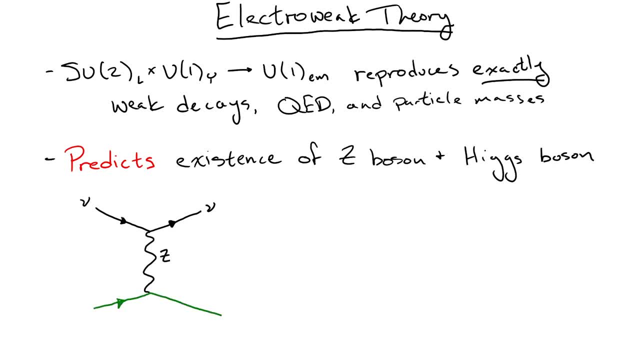 After the formulation we have the Higgs boson. In other words, we've already taken the Higgs boson of the Higgs boson matrix over the Higgs boson. Now let's go back to the calculation of electroweak theory.